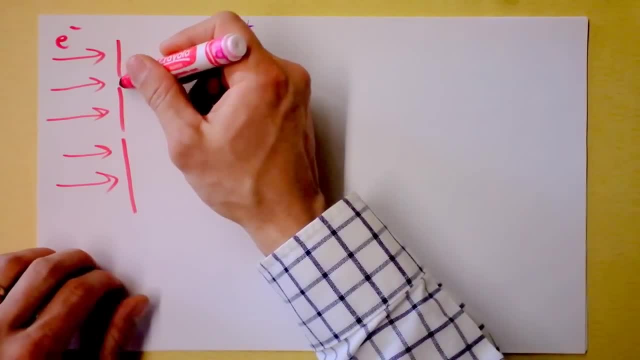 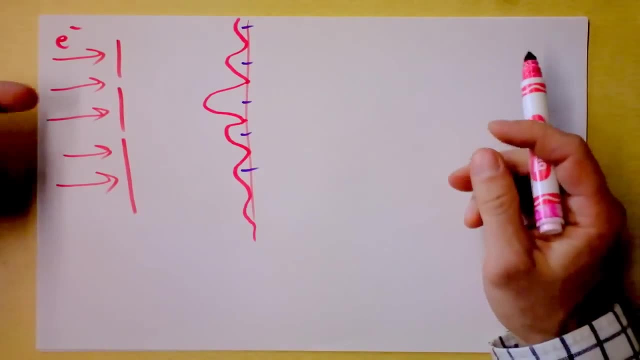 going to go when it gets through here, because it's as if they are bending as they reach this point right here. there's nothing exerting a force on them, though it's not like there's a magnet there that's turning the electrons or something. it's that by confining them to go through a slit. 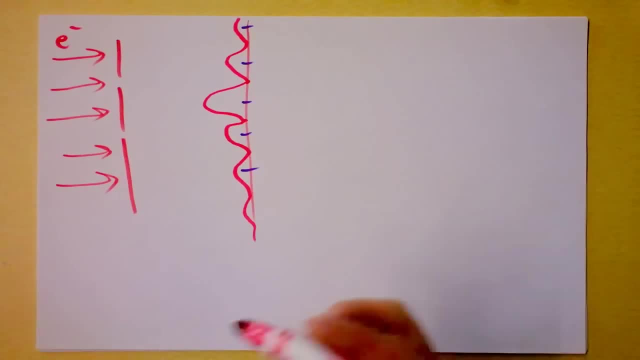 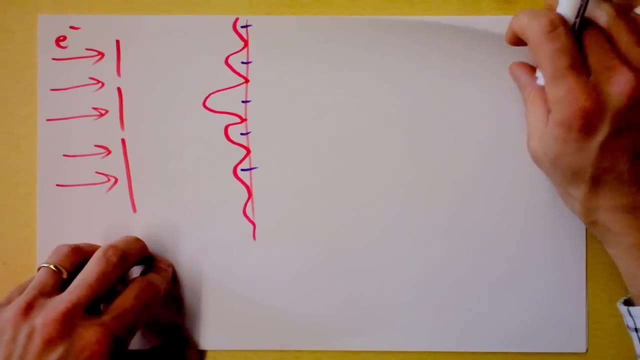 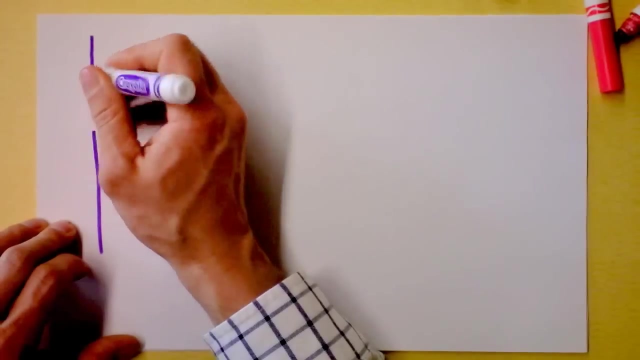 there's some uncertainty introduced into which direction they're going, so let's develop that a little bit further. um, i'm going to go to just a single slit and on this single slit let's let's take another uh sheet entirely here. i have electrons coming in over here and the width of 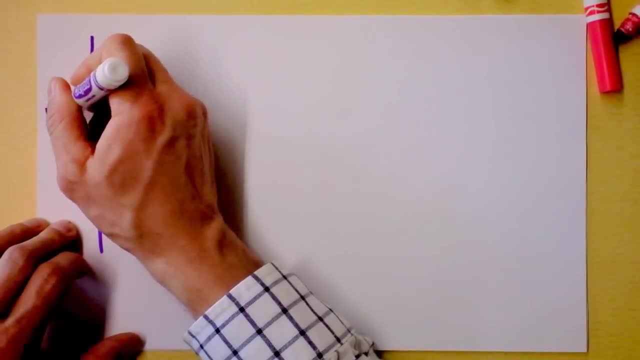 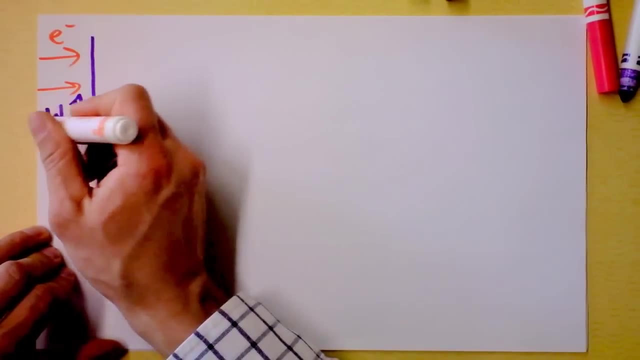 the slit will be defined as w. let's set this up and then send some electrons in. my electrons will be orange, orange, orange. this time electrons are coming in this direction and i don't care if you send them in one at a time, but many electrons will hit the wall, but the electrons that make it through do eventually. 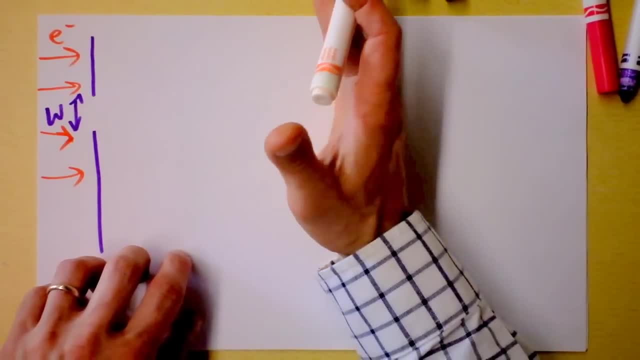 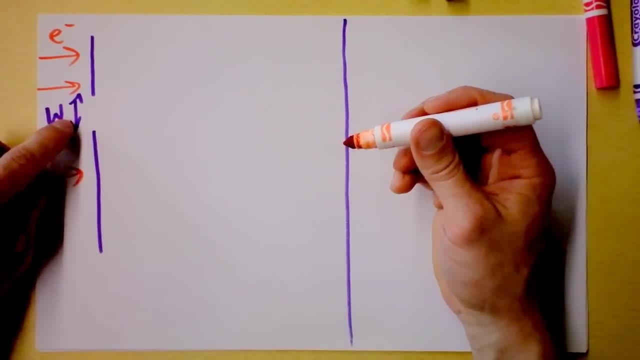 appear on a screen that's going to be i don't know. let's put it right here so we can do a little bit of math. also, let's make the screen purple and since the electrons are orange, we're going to say that there is a bright fringe. remember, with the um, with the single slit diffraction, you should. 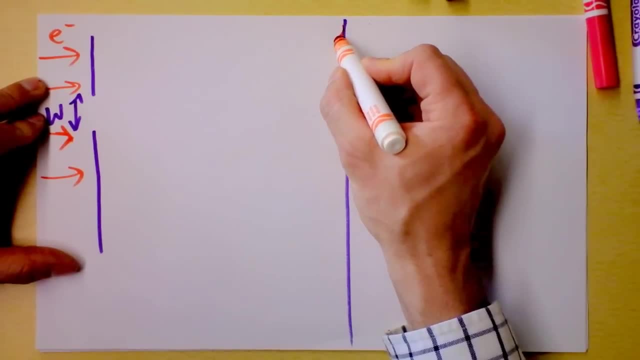 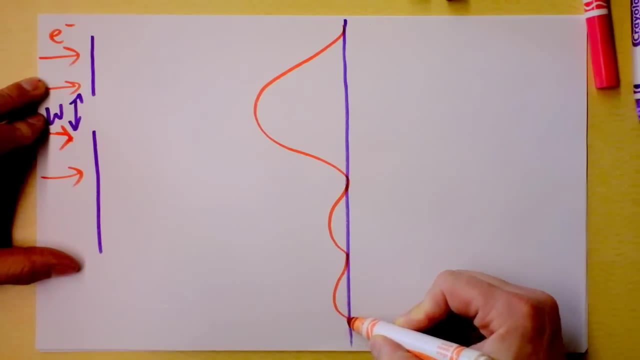 review that, if that's not something that you remember easily. with a single slit diffraction we have a very wide central fringe and then we have other bright fringes and we're not going to talk about them, but they're a little bit narrower and they taper off like this. i'm interested in primarily the wide. 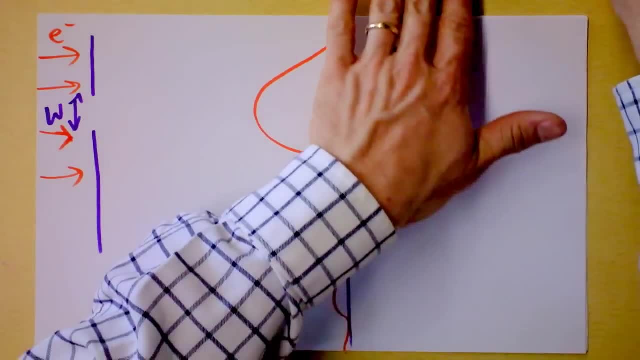 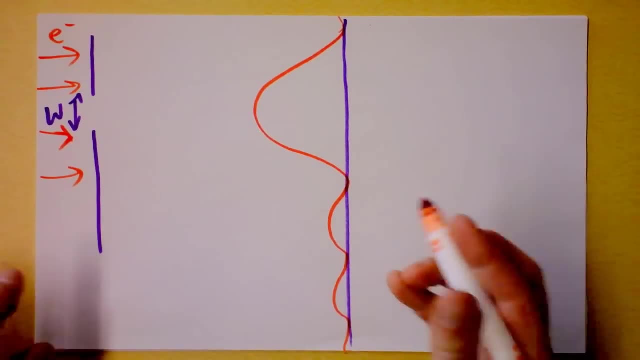 central fringe. this is the sloppiest derivation of the heisenberg uncertainty principle that you will ever see. if you want to see it in more detail you'll have to look in a deeper physics class. but my introduction right here is just going to tell you kind of a feel for the heisenberg uncertainty. 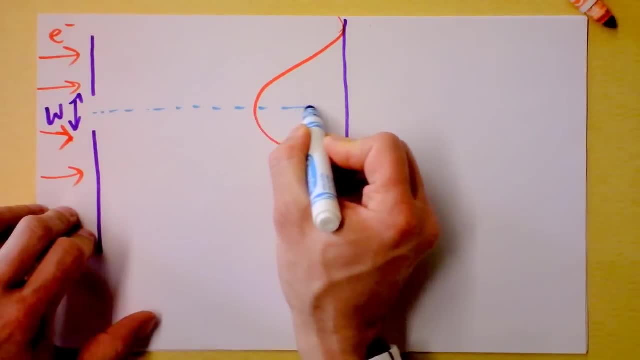 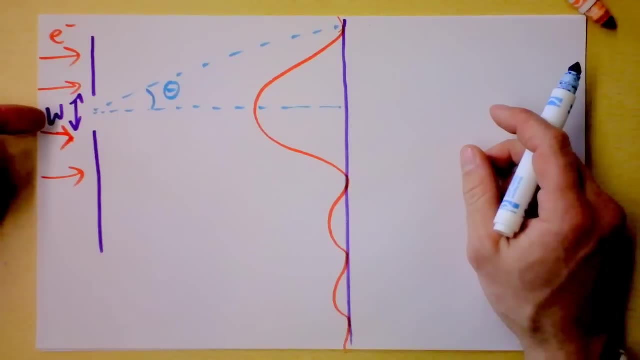 principle. i'm frankly happy that we can even do this much. so there we go, and then i'm going to give you an angle, and then i'm going to give you an angle, and then i'm going to give you an angle here, theta, and i guess what i'm saying is: when an electron goes through this slit, it will appear. 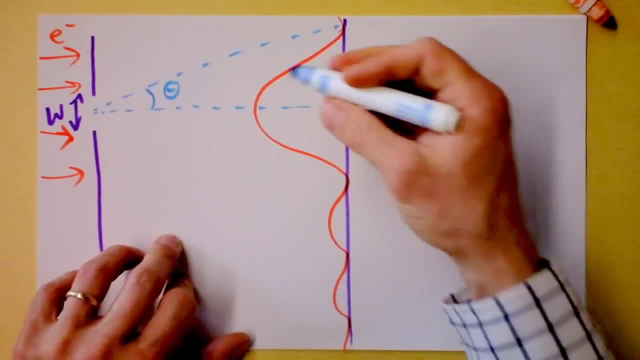 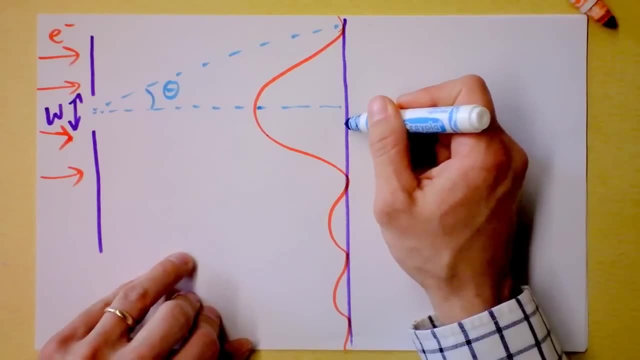 somewhere there is a bright fringe. so if it might appear here, there's a pretty good chance of it appearing right there. but there's also a very reasonable chance that it might appear here, i mean here on the screen, here on the screen. this is maybe the most likely place for it to appear. 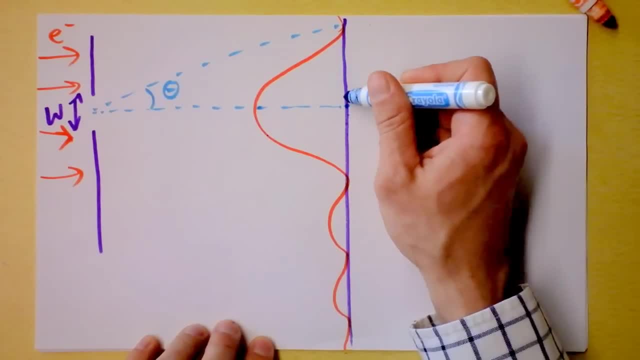 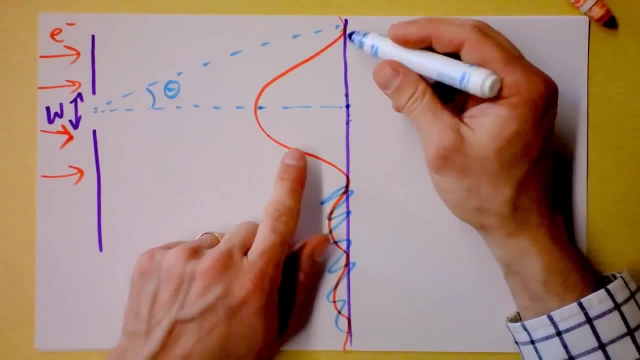 but way fewer than 50 percent of the electrons appear right here. you got some appearing here, some appearing here, some will even appear here. but remember, i'm going to disregard those guys right now. i'm going to say that there's some chance that the electron will. 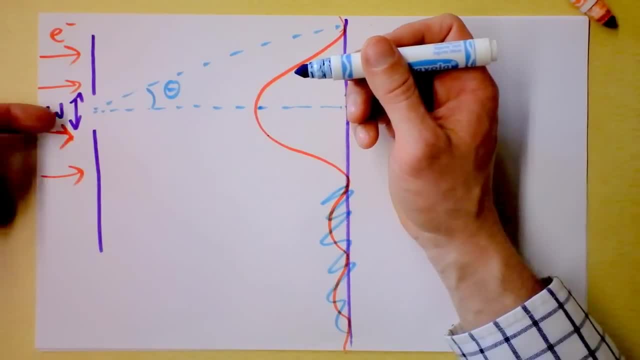 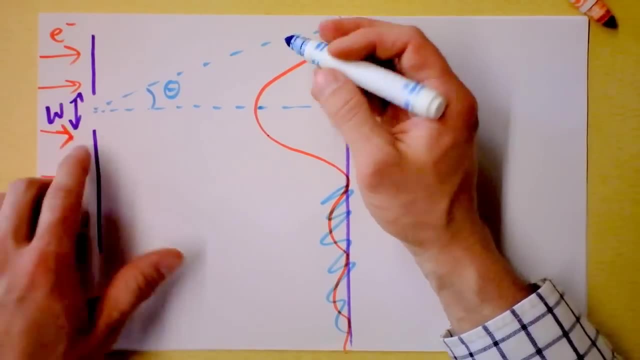 fall right in here. it's most likely to fall somewhere in the middle because, remember, they're all lined up exactly, they're all coming in exactly horizontally. so you would think, if it were just classical physics, that they would all appear at this point, right here, because they're all pointing. 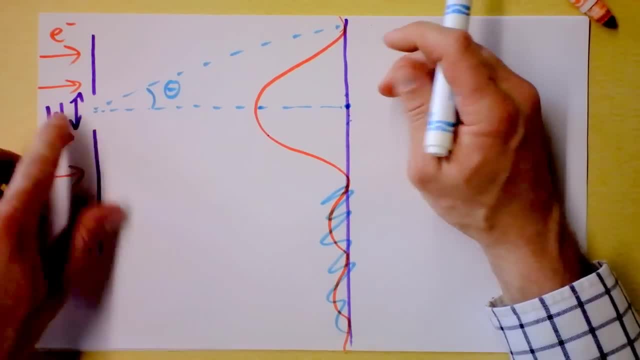 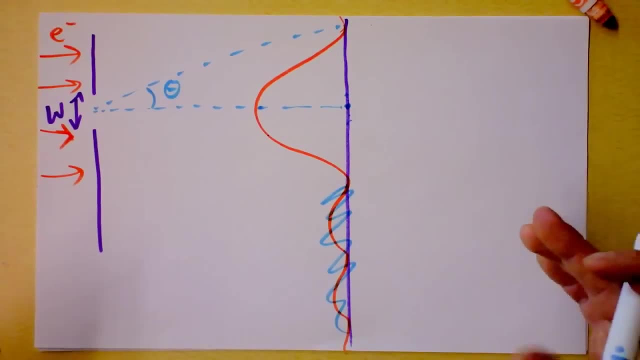 exactly straight, or maybe just a width of w, but this is way wider than w, depending on the angle. there's a spreading because of diffraction, so electrons are interfering with themselves. i want to first define where that dark fringe is. remember, for single slit diffraction it's as if there are two little double slits. i'm 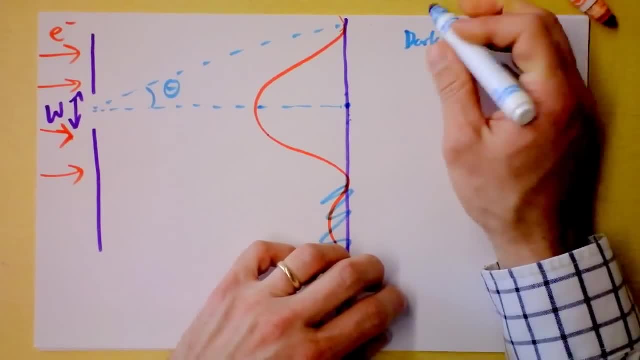 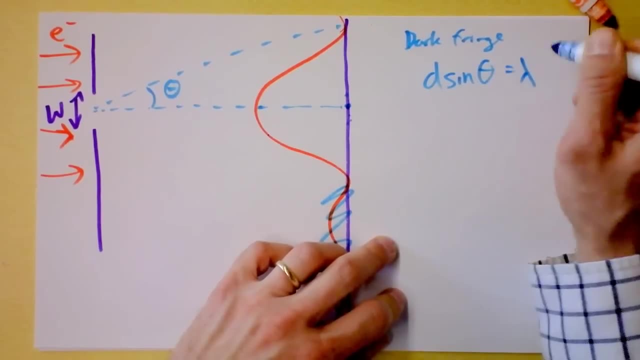 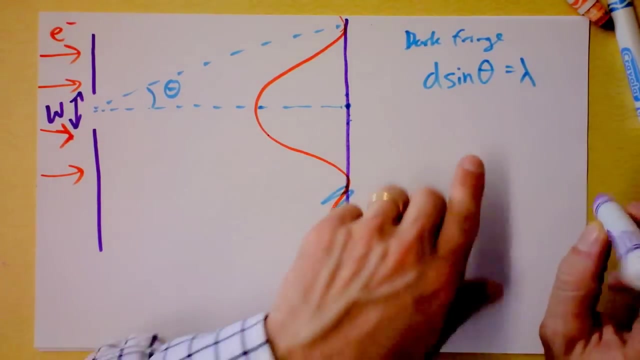 not going to go through that, but i'm going to tell you that a dark fringe appears here. my dark fringe is at d times. sine of theta is a wavelength and we're talking about the wavelength of the electron, so we're fully quantum here. this might be a huge headache for you, i don't know, but i'm okay saying: 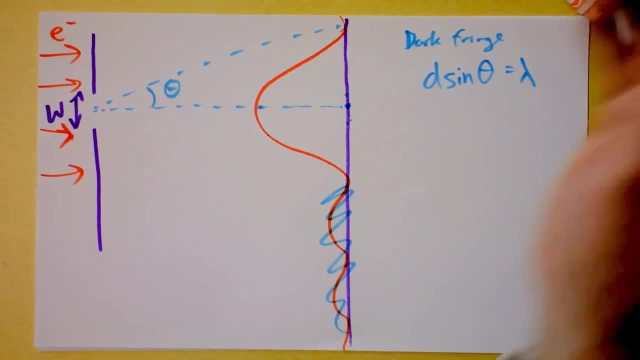 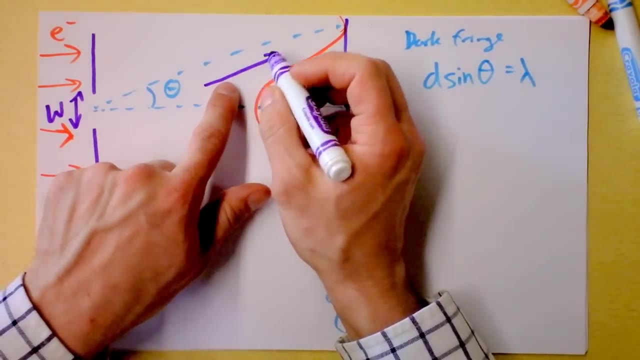 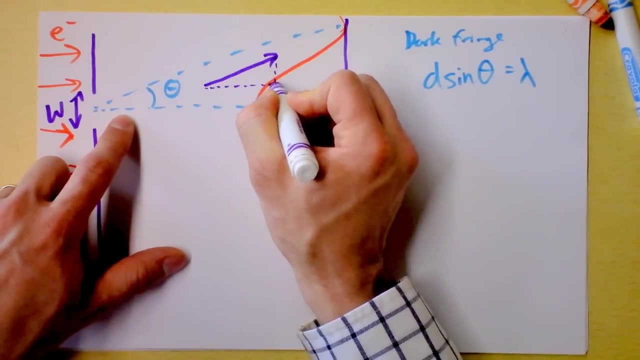 that the dark fringe is at, where d sine theta is the wavelength of the electron. and i'll present to you some vectors. and this is the vector of: well, this is the overall momentum of an electron that just makes it to the edge right there, and then i can define these two components of that vector. well, this guy here is. 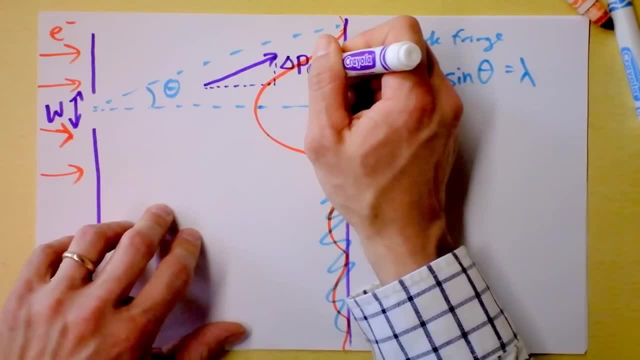 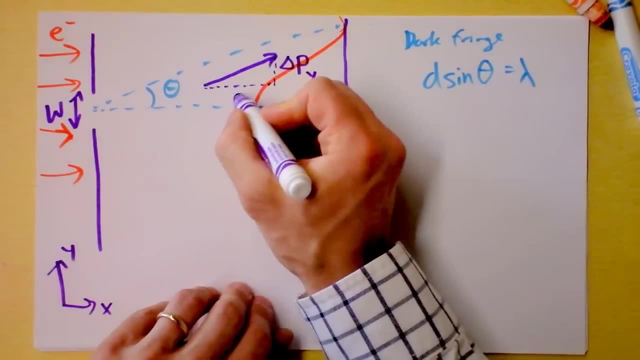 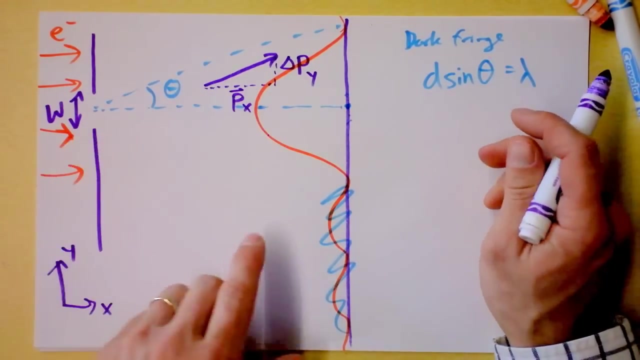 going to be the. i'm going to call it delta p in the delta p in the y direction. so i need to set up my axes. i've got x here and y here and i'm going to call this the momentum in the x direction. we know it has momentum in the x direction and nobody is saying that there's any weirdness in that. but 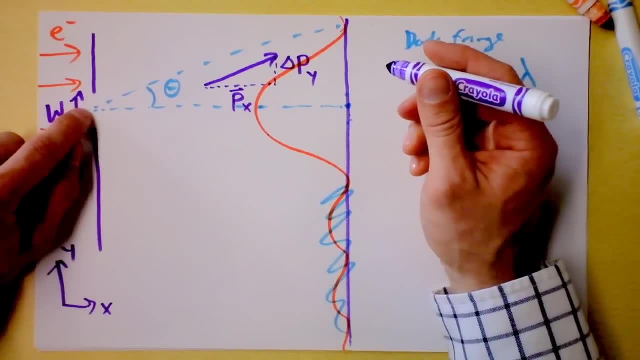 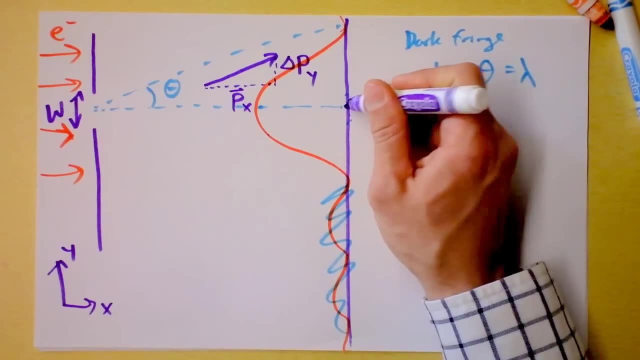 i'm saying that as soon as the electron goes through this slit, you don't know which way it's pointing in y, you don't know what its momentum will do in y. it may get no momentum in y and then hit right here. it may get some momentum in y and hit up here, or some negative momentum in y and hit. 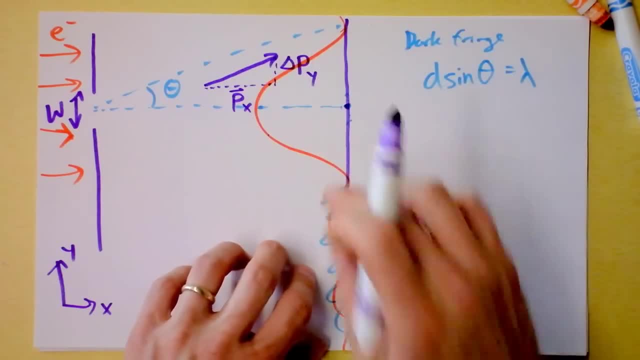 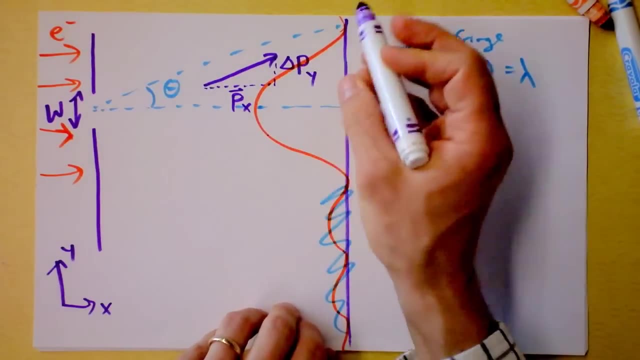 down here this: the fact that there is a wide fringe, means that there is uncertainty in which way the electron is going in the y direction. so i don't want you to think as of this as change in momentum in the y direction. that's how we used to write deltas, but i'm going to call it delta p in the y direction. 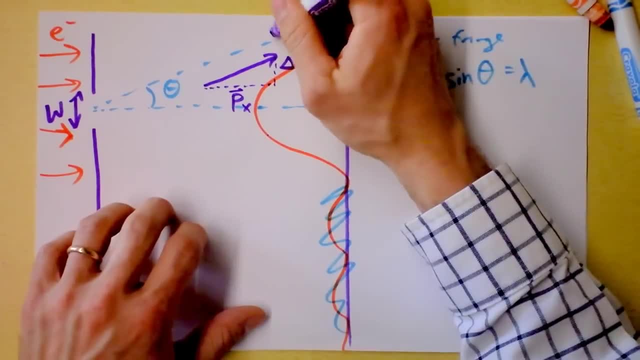 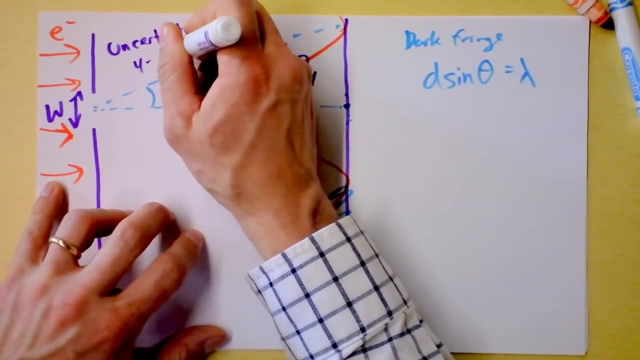 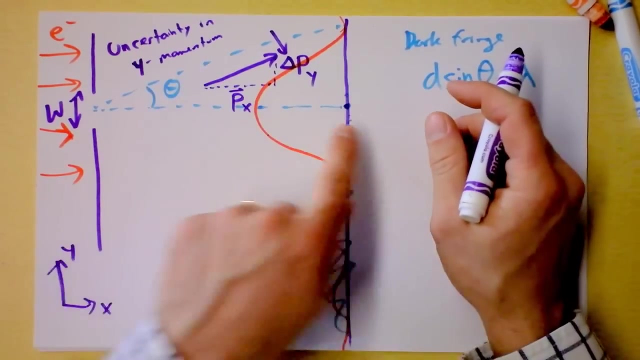 this is uncertainty and momentum in the y direction. let me actually label that uncertainty in y momentum. now let's think about uncertainty in position. there is some uncertainty in the y position at this moment, right here. we don't exactly know where the electron is inside of this. 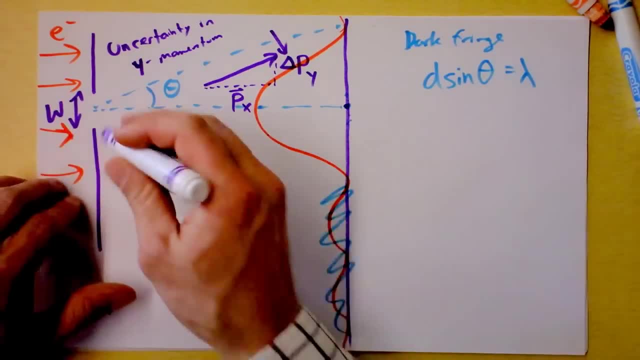 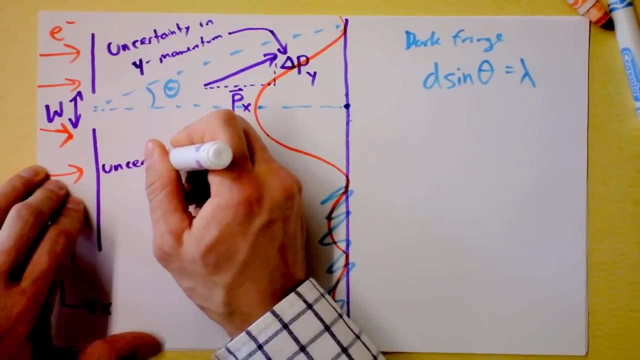 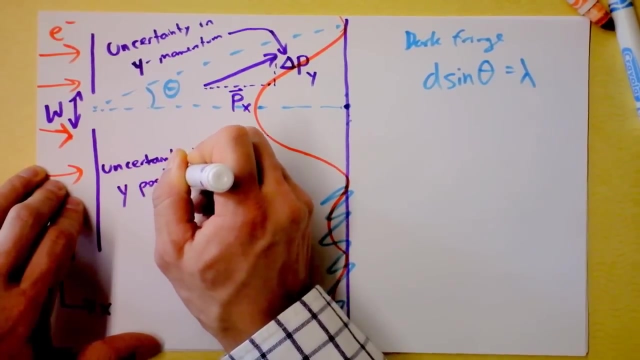 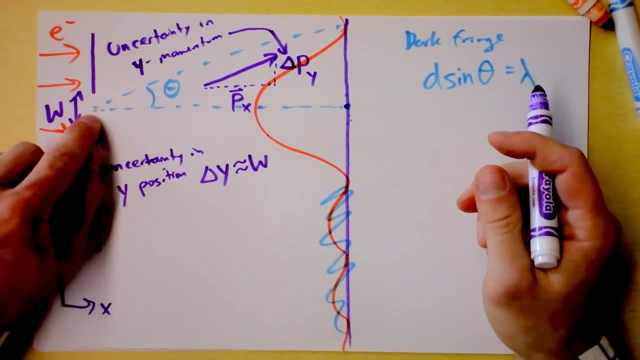 slit. we kind of think that it might be a lot of places because it's doing some quantum stuff. but the uncertainty- i'm going to label that as the uncertainty in the y momentum, uncertainty in y position- is delta y and that's kind of like: w do you notice that? we really don't know whether it's gone here, here, here, here, here, here. so 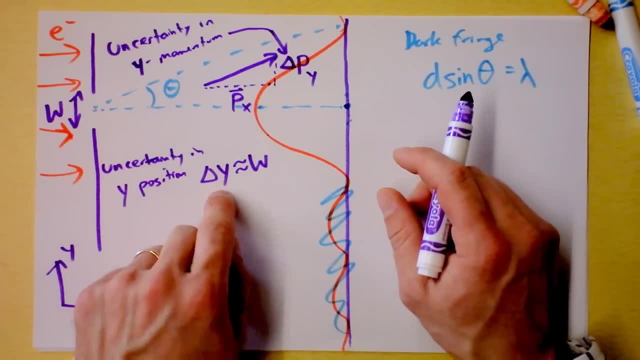 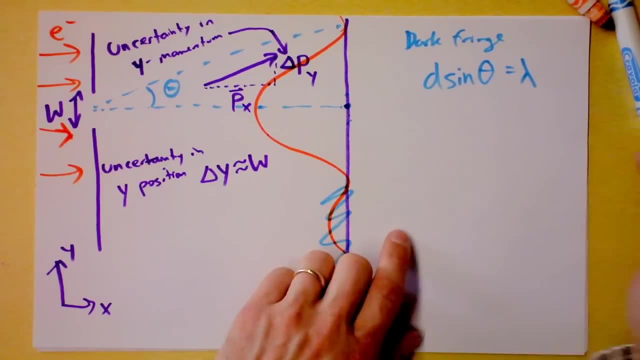 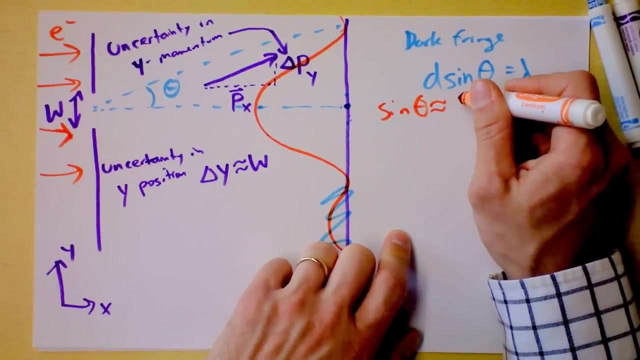 there's some uncertainty in the y position as it enters this single slit apparatus. so here's my plan. i can rearrange this just a little bit and find that the sine of theta- let's go orange for this next line. the sine of theta is approximately equal to: 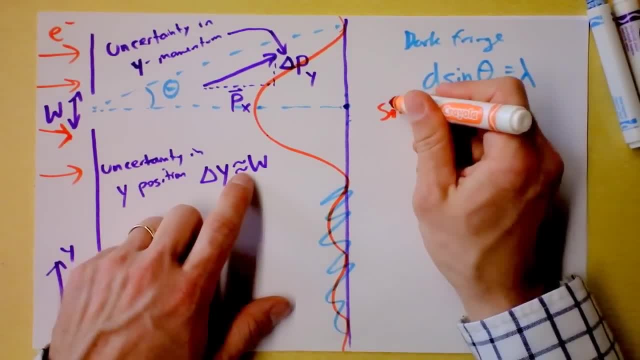 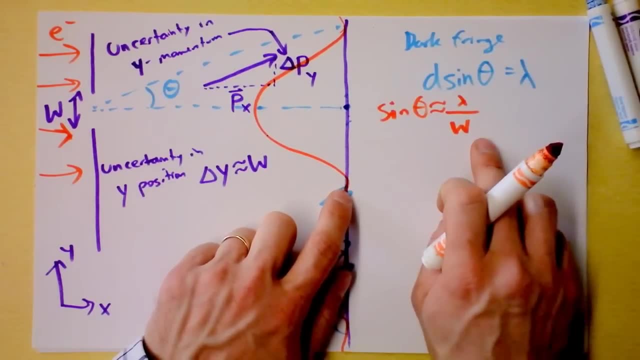 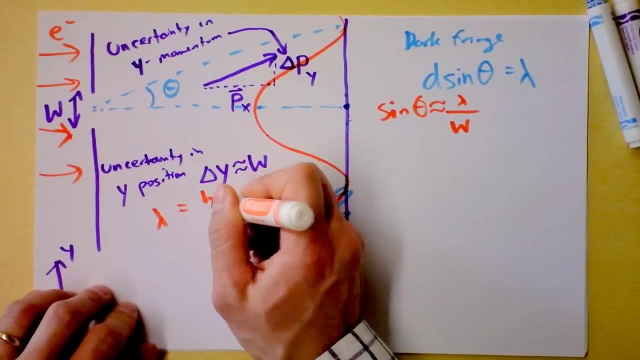 lambda divided by the width of my slit. okay, so that's all right. that's all right. so there's a little bit of uncertainty here. dark fringe, dark fringe, and in between those two dark fringes we've got the width of our central fringe. now you remember, of course, that lambda is h over p sub x. this is de broglie who says that, that if there's a 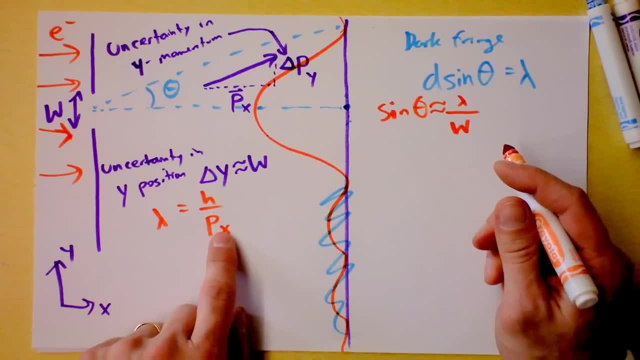 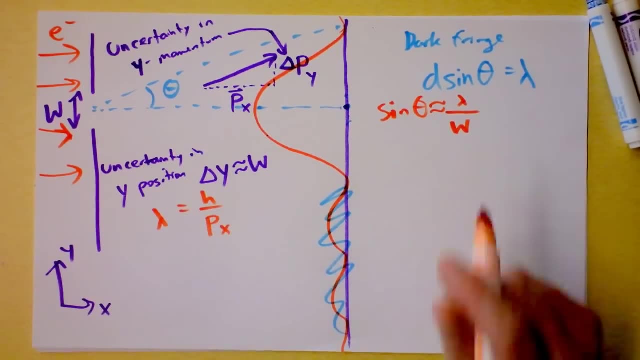 uncertainty. well no, that's not what he says. he's saying that if there's momentum, and there is momentum in the x direction, then there is a wavelength, and that wavelength is defined by h Planck's constant, divided by the momentum right there. so here's what i'm saying: this electron beam. 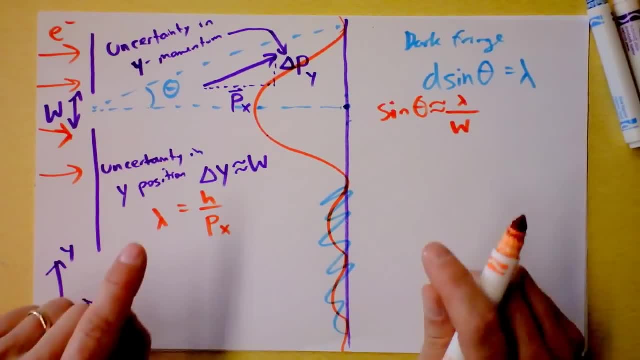 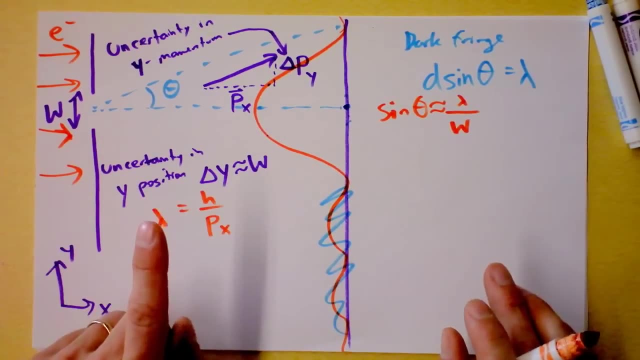 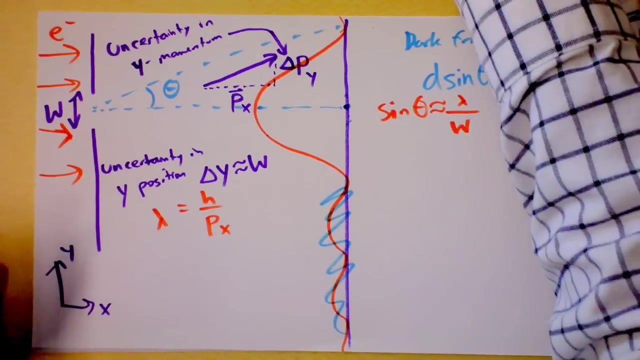 spreads out in a diffraction pattern, which means that the electron has momentum uncertainty, and i'm going to say the momentum uncertainty, ooh. can we talk about this? can we talk about how the width of this slit will affect the uncertainty over here? i think we should do that. consider, if you will, a slit that is very, very. 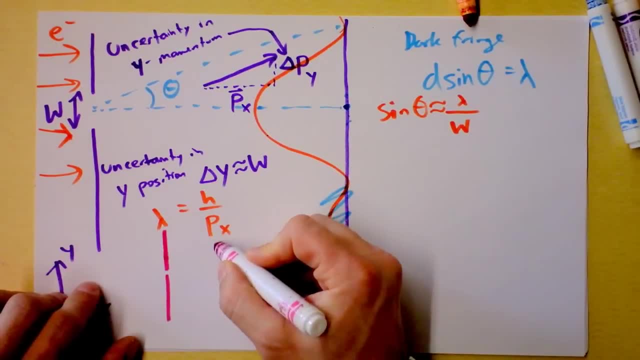 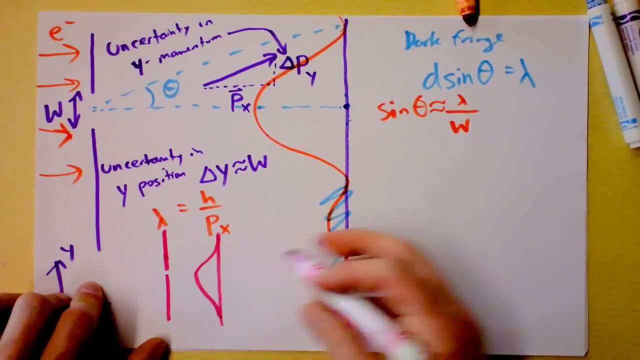 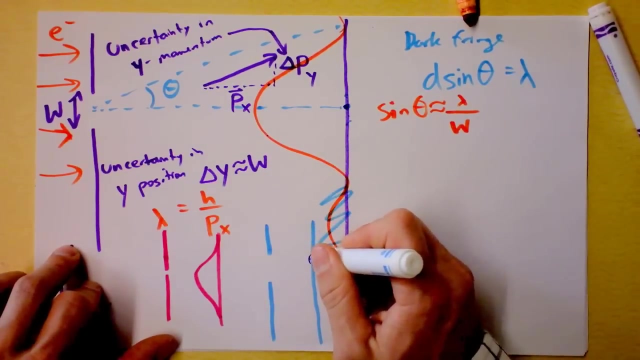 narrow. do you remember what the fringe pattern for a very narrow slit looks like? oh yeah, it's really spread out. and what if i have a slit pattern that is very, very wide? well, if it's a very wide slit pattern, then we don't have as much diffraction, or maybe what i mean is these are closer together, so we're actually going to get a. 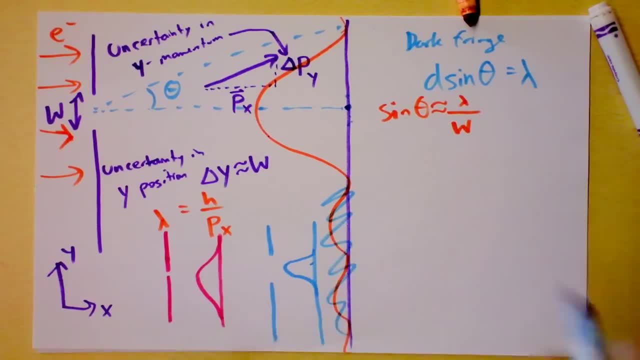 much narrower peak as a result. This is very counterintuitive, but go back and look at how diffraction works and you'll find that a well, the better, ooh, the better we know where this electron was, the worse we know which way it's going: up and down. The- oh, look at this. The. 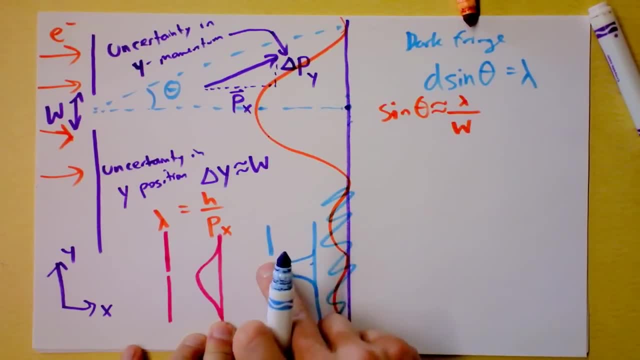 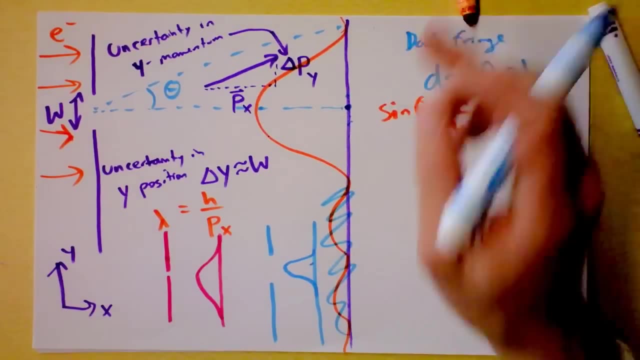 worse we know about where the electron is up and down, the more accurately we know how fast it's going up and down. This is very interesting. There's like a trade-off, Like you get to know one thing but not the other. So let's go back here and do a little bit of math, a little bit. 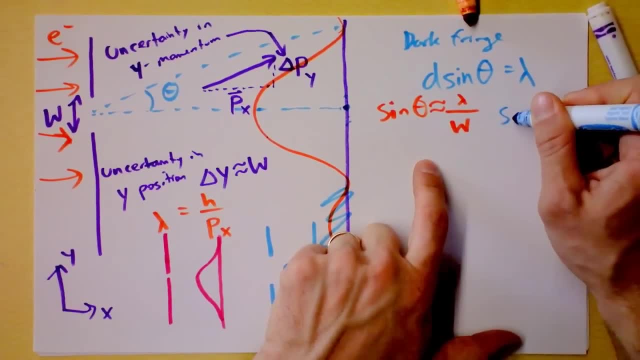 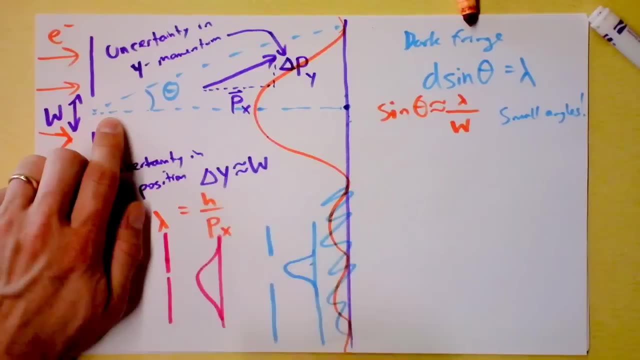 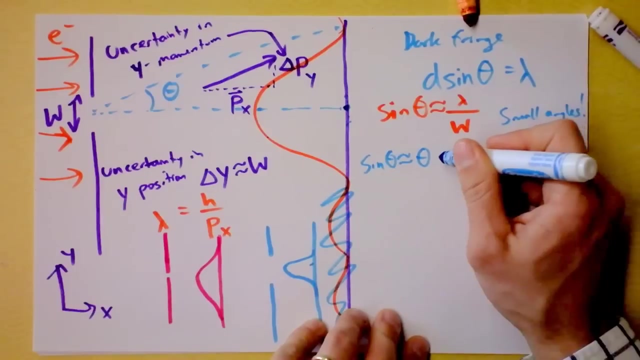 more careful. I want to use the small angle, approximation, small angles, And I'm going to say that that means the screen is very, very far away. So we have a small angle for the width of that peak right there And I'm going to say that sine of theta is approximately theta And I'm 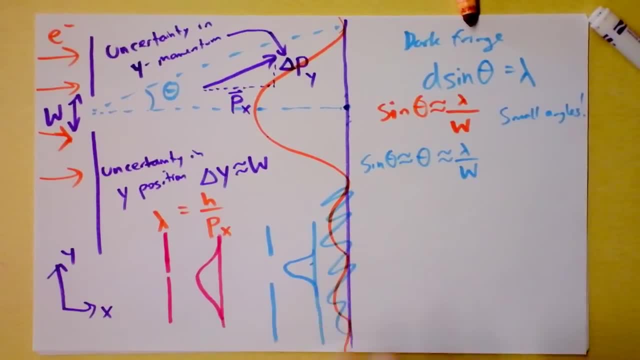 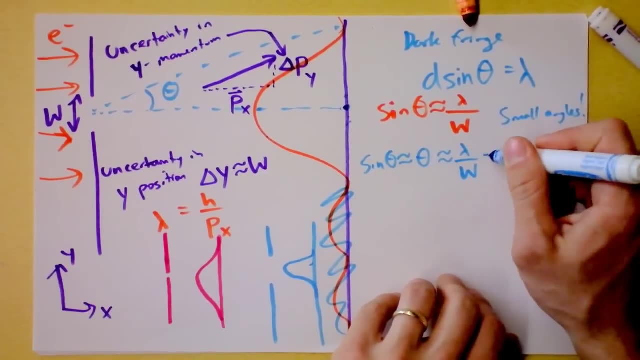 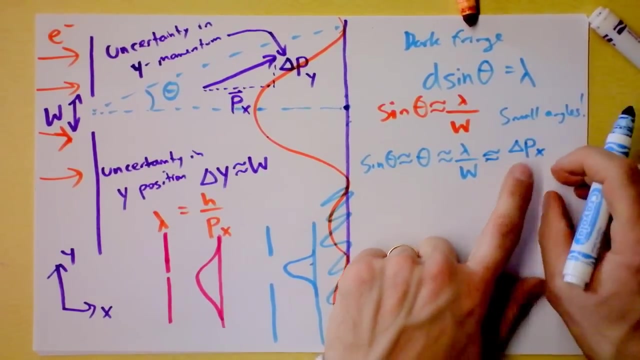 saying that theta is about lambda over the width of the slit. But what I'm about to do, watch this. I'm about to say that this is well, it's kind of about. also, it's going to be delta P Y. Remember, this is delta P Y, right there, divided by P sub X, Did I? 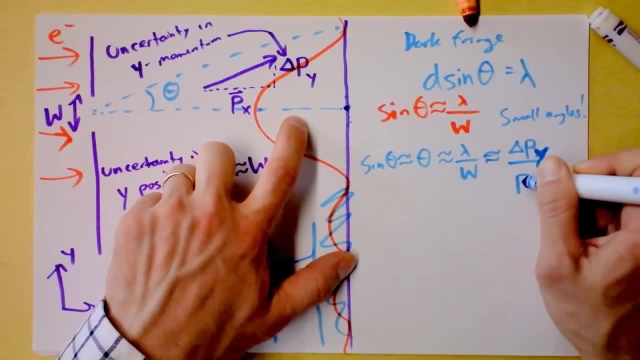 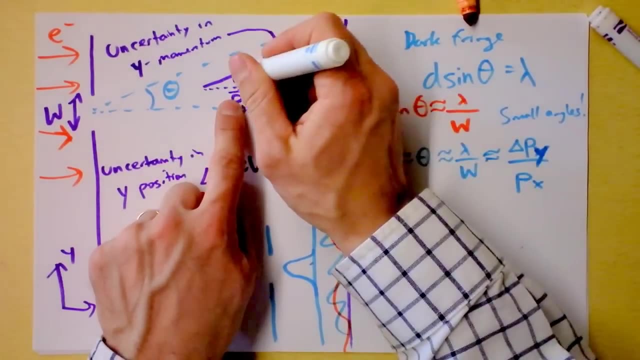 make an X there. Sorry, Delta P Y divided by P sub X, because the sine of theta is pretty much the tangent of theta. So I've got opposite divided by adjacent And for small angles, same angle, theta right here, sine of theta and tangent of theta and theta are all pretty much. 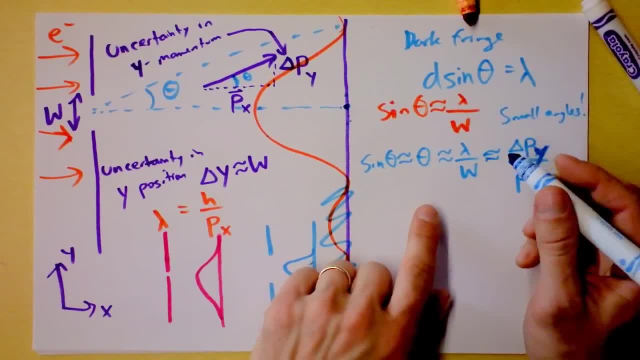 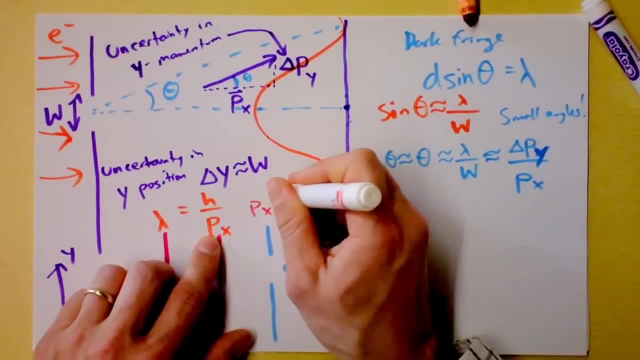 the same thing. I've done that in a few videos. I'm not going to do that again for you today. We've got two definitions that we need. I'm going to solve this equation for P sub X first, And P sub X is H over lambda, And I'm going to take that That's a lambda, not an X. P sub X is: 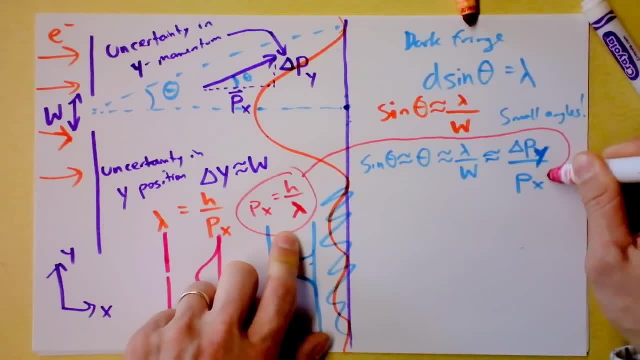 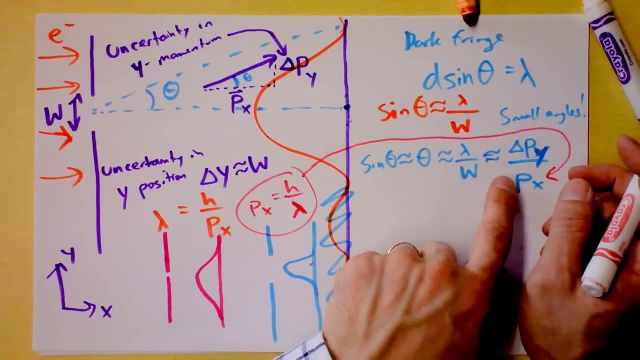 H over lambda. I'm going to plug it in right here. Watch me put it right there. And the other equation that I need is an equation for the width being about delta Y. Oh no, I've already put that in there. No, no, let's do that. 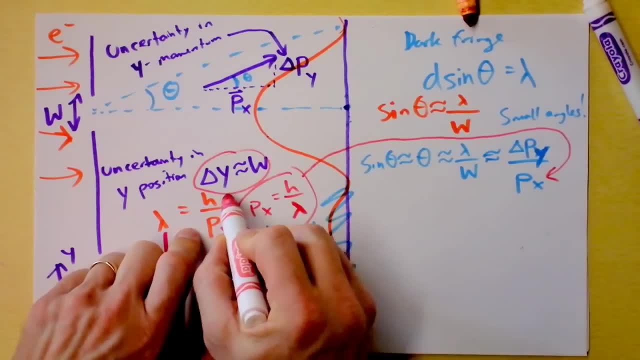 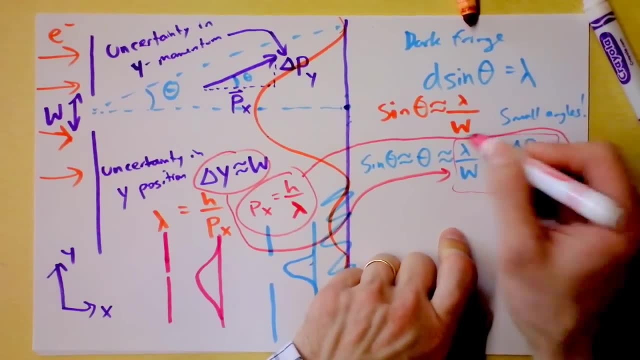 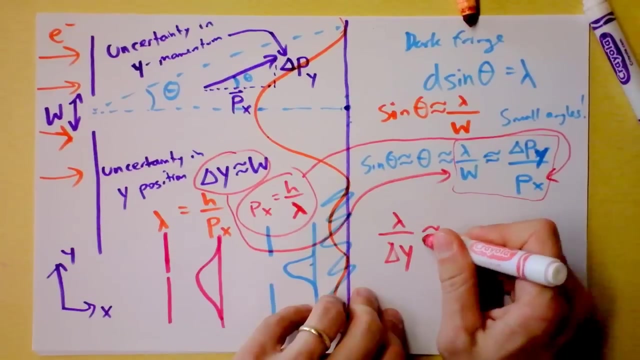 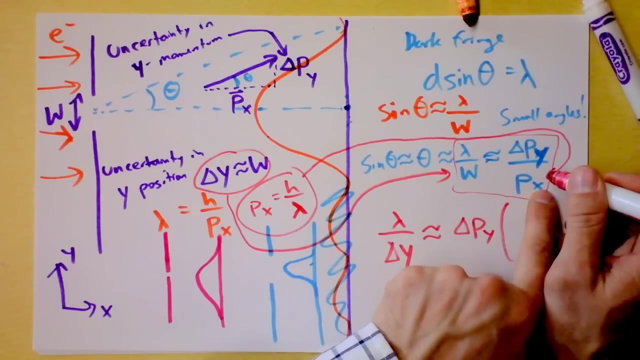 Let's say that this equation is going to go in here, And so my equation- then what was right here- will be rewritten as lambda. divided by delta Y, because that's my W- is approximately. well, it's going to be delta P, Y, And then I have to. well, I'm going to divide by P. 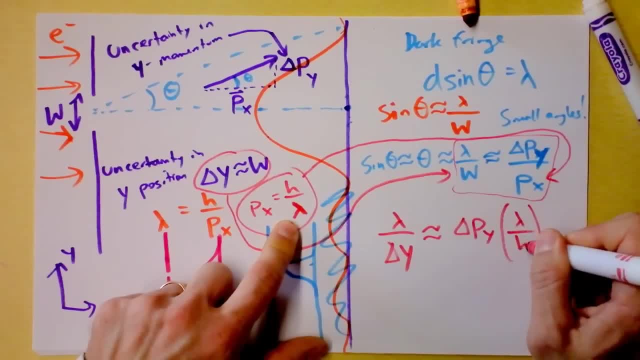 X. So I'm going to write the inverse of this sucker here. It's going to be lambda over H And if I rearrange these guys canceling out my lambdas, that's fun. Cancel, cancel, Then I get. 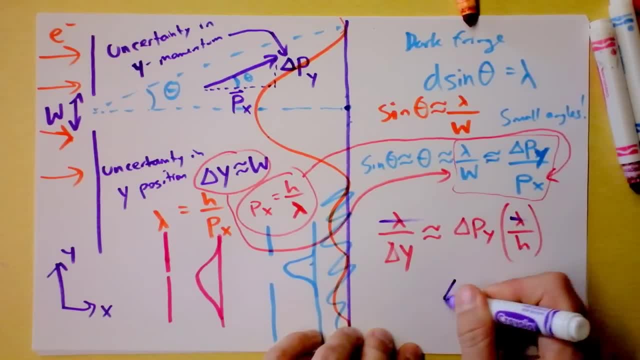 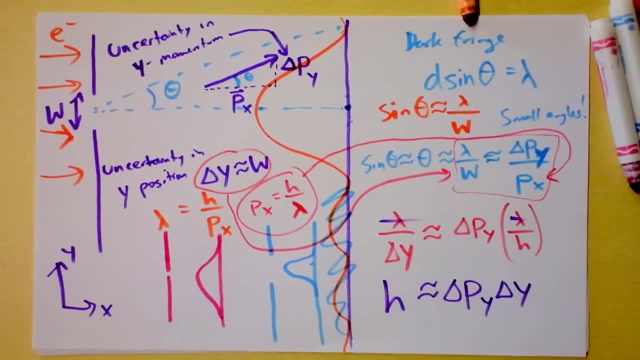 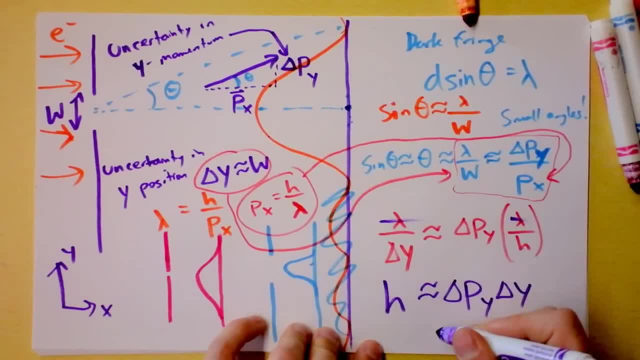 I'm doing this stupidly. you'll say that's not exactly what it is, Dr Schuster, And I'll say you're right. In fact, this uncertainty in the momentum in the Y direction, multiplied by the uncertainty of the 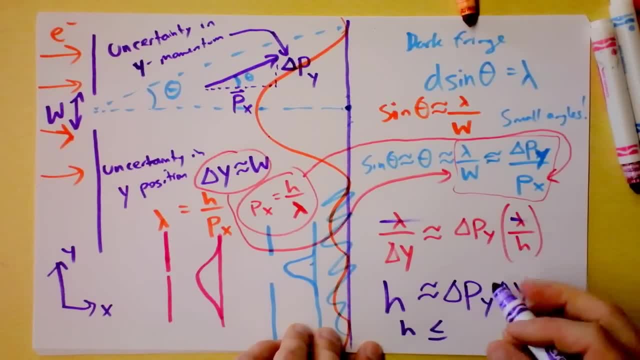 position in the Y direction has to be greater than or equal to 2 pi. H divided by 2 pi. So I've got delta P Y times delta Y, And a more formal treatment will get you this result right here. That is the Heisenberg uncertainty principle, And a lot of people write H divided by 2 pi all. 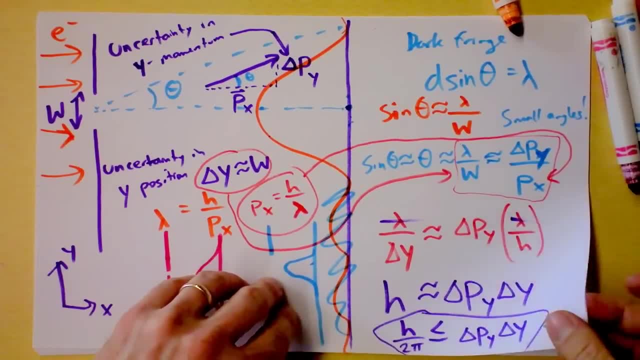 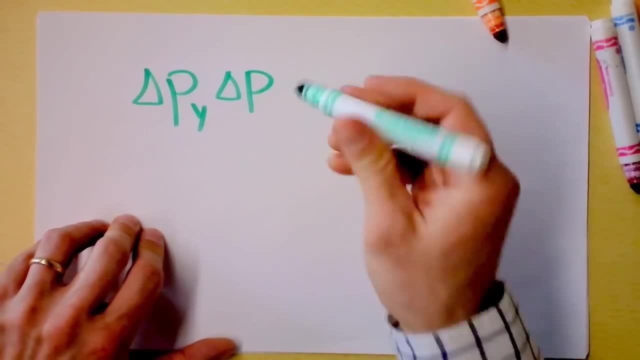 the time. So a lot of people will write: well, what's the Heisenberg uncertainty principle? like this: They will say that the uncertainty in momentum in the Y direction multiplied by the uncertainty. Ah, that's not what they'll write. 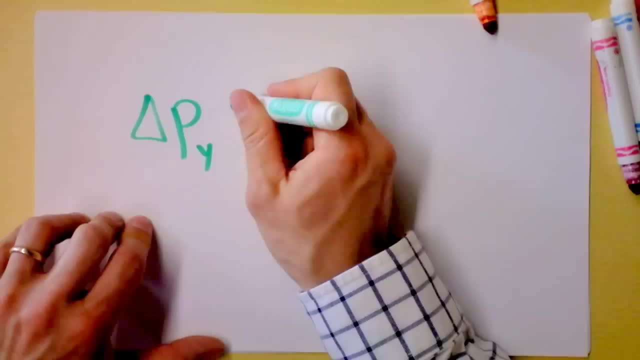 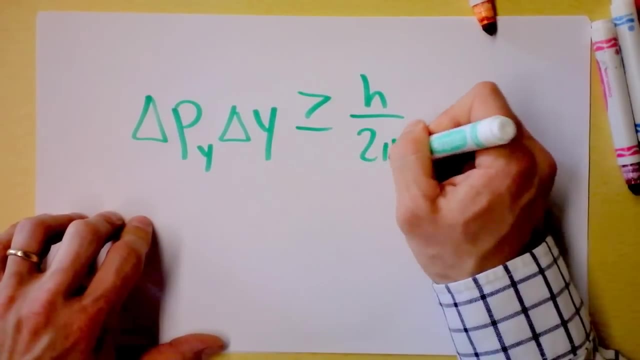 Dang it. The uncertainty in momentum in the Y direction multiplied by the uncertainty in position in the Y direction has to be equal to or greater than H divided by 2 pi, which is just H bar. That means divided by 2 pi. It's a cool symbol. You can write all sorts of things divided. 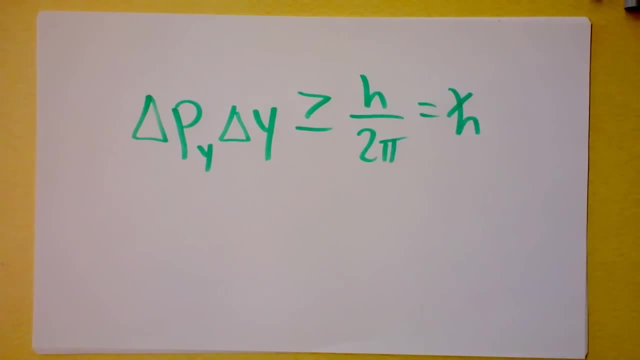 by 2 pi by just putting a little slash in there. So I'm going to write delta P Y times delta P Y. I'm putting a little slash through them Like they're canceled, but they're not, They're just divided by 2 pi. So this is really really really deeply awesome. Heisenberg's wife would. 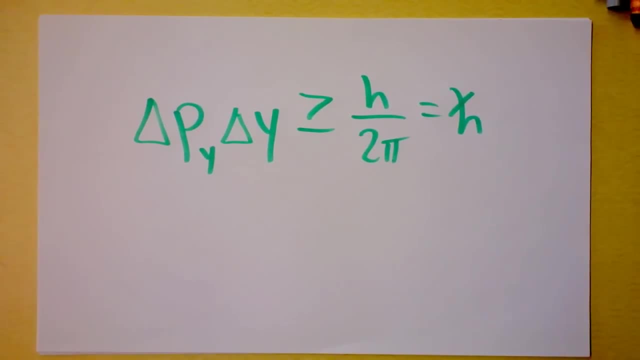 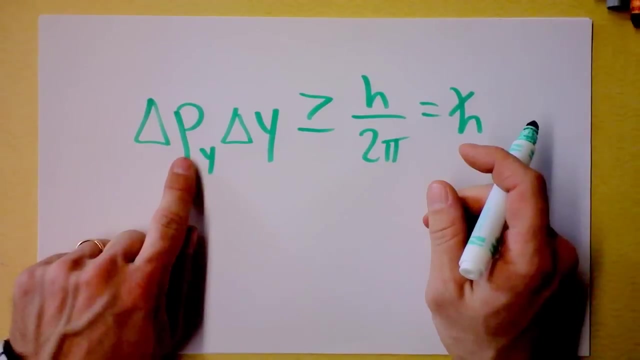 lose her keys from time to time and she would always say to him: honey, I don't know where my keys are. And Heisenberg would respond: sweetie, it is likely that you know far too much about their velocity. You see, momentum and velocity are just proportional to mass, related by mass. 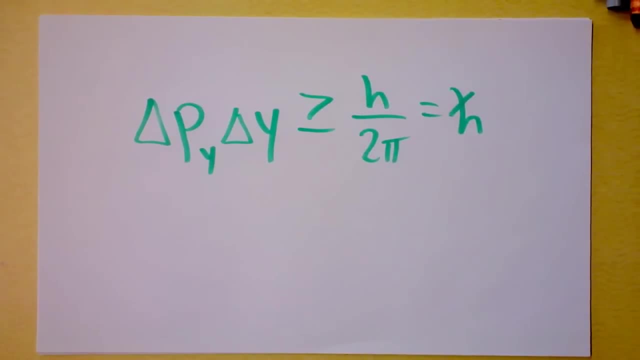 So if she knew- oh man, that's funny, Shut up. I'm not going to explain that to you, That's a joke- Or the cops would pull over Heisenberg sometimes and the cop comes up to him and he's. 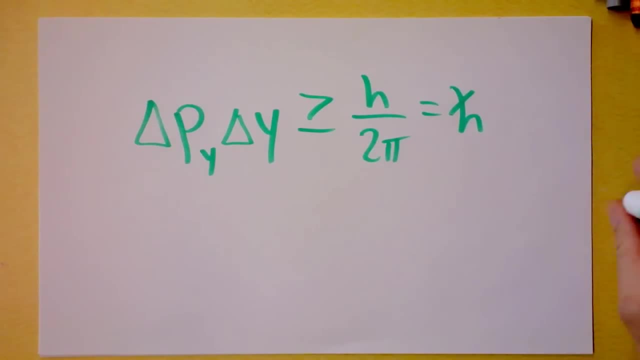 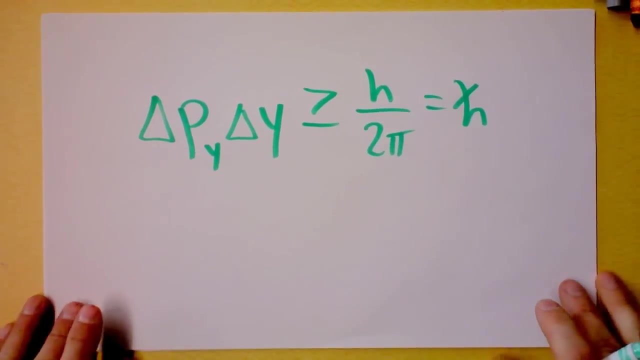 like Professor Heisenberg, do you have any idea how fast you were going? And Heisenberg says no, but I knew exactly where I was. Ah, so good. Now that's all well and good, but here's another. 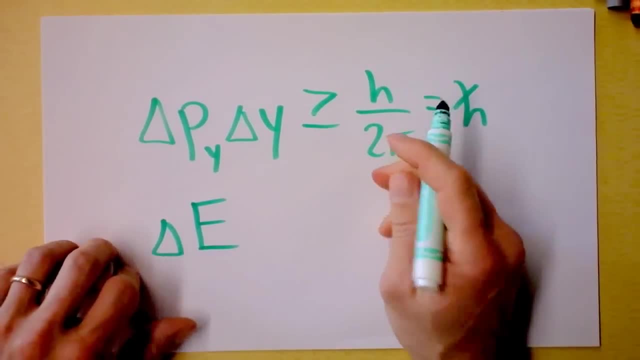 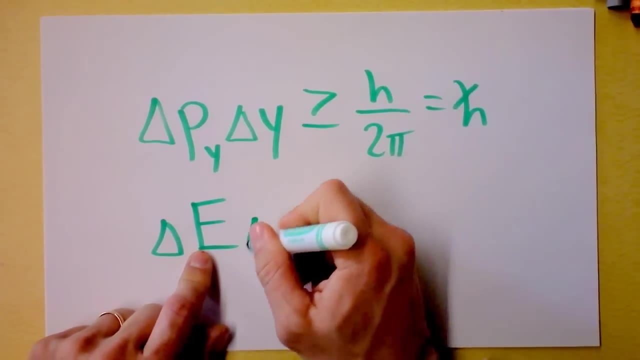 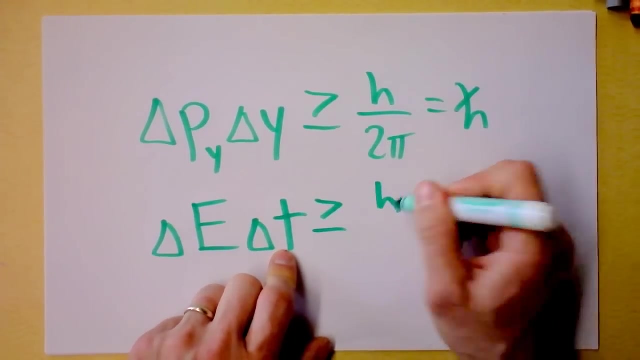 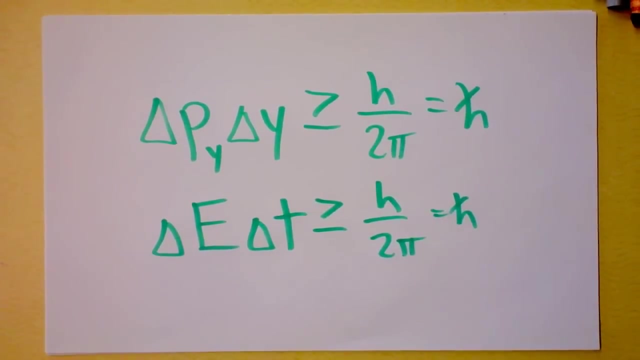 here's another uncertainty equation that can be derived in a similar manner. different experiment, probably. So I'm saying that the uncertainty in the energy of a system, multiplied by the uncertainty in the time that you take to measure that energy, is also always greater than or equal to h divided by 2 pi or h bar. Oh, my goodness, You're saying that, if I don't. 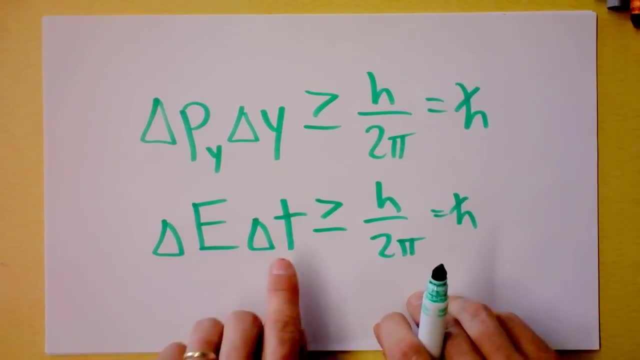 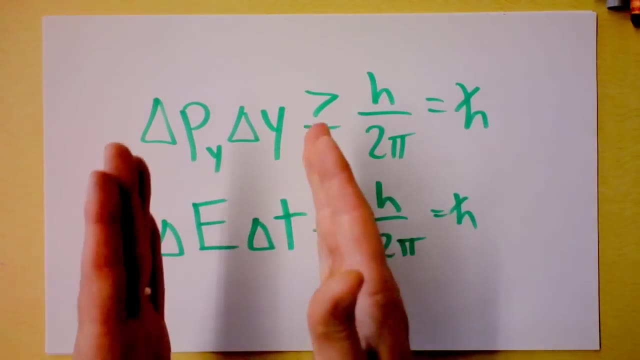 spend very much time measuring a system, I can't tell what its energy is If the time uncertainty is very big. ooh, I guess that's what I mean. If I measure a very, very accurate time, then the time uncertainty is very small, then the energy uncertainty will be very, very small. And if I measure a very, very 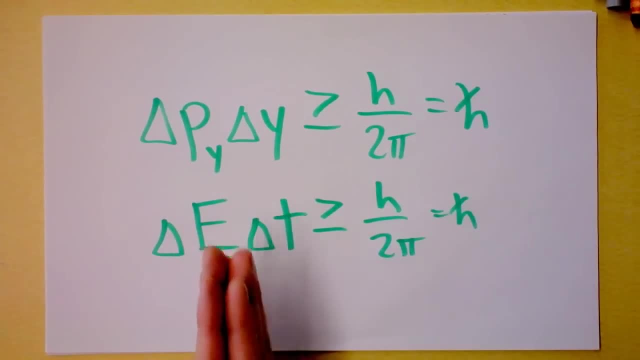 big, in fact, at smaller and smaller time intervals. that means you're getting more and more accurate knowledge of the time. If you are measuring at a very, very, very, very small interval, you have, frankly, no idea how much energy a system can have. And looked on short time scales, you get stuff. 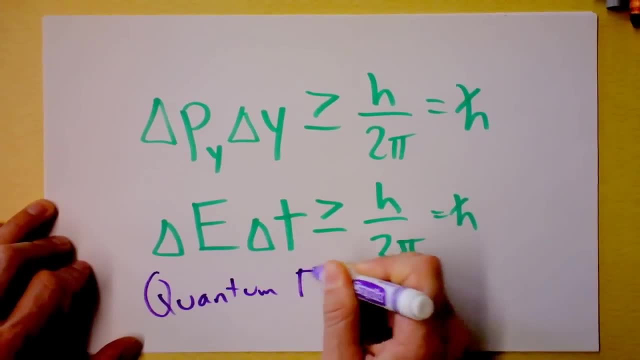 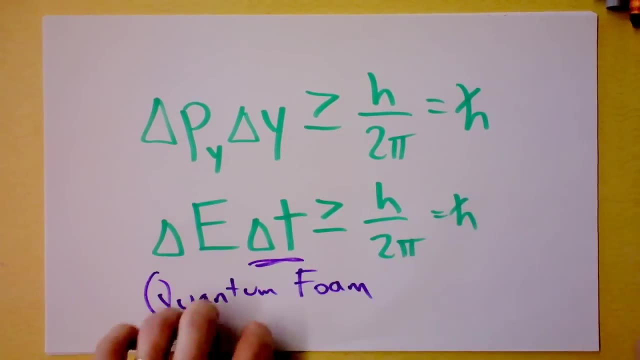 called quantum foam. That's pretty cool. Quantum foam is stuff that pops into existence and out of existence very, very rapidly, because this time uncertainty is incredibly small, so the energy uncertainty has to become incredibly big. This is a fundamental uncertainty. It talks. 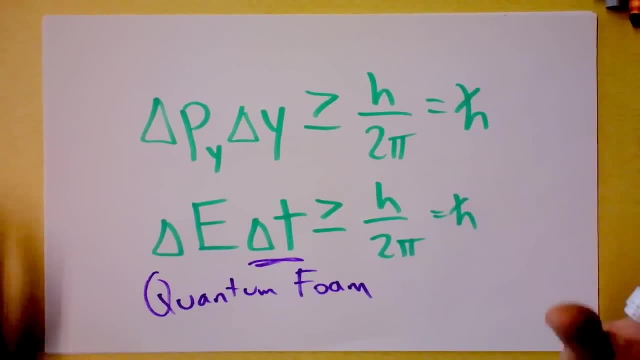 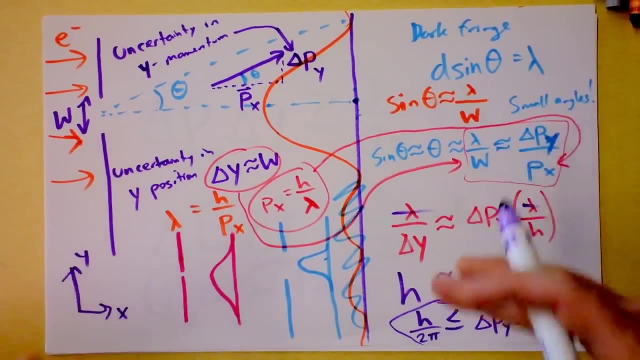 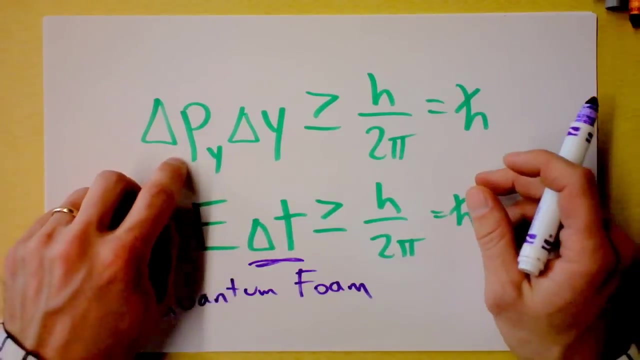 about what can be known and what can't be known about the universe. There's no way to circumvent this. This example of electrons going through a single slit is simply a way to derive it, but it applies to everything all the time. If you know one thing too accurately, then you're 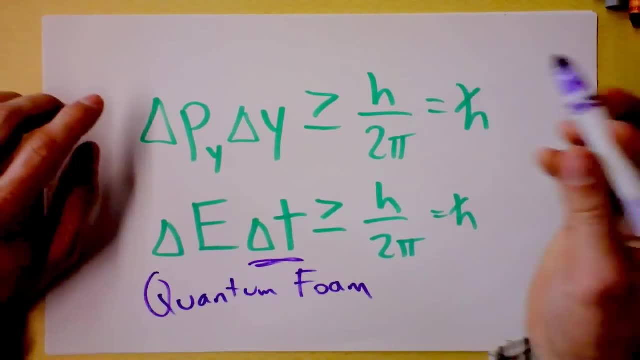 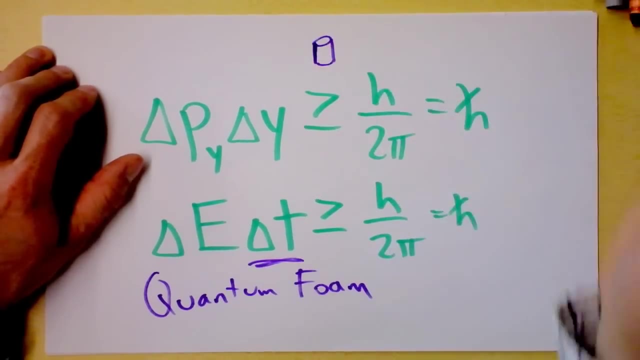 fundamentally screwing up. another thing. I like to think of it like this: You know that there might be, I don't know, a can of Campbell's soup right here, but it's extremely, extremely small, Like, let's say, it's an electron or something. So there's an electron right here and the electron you want. 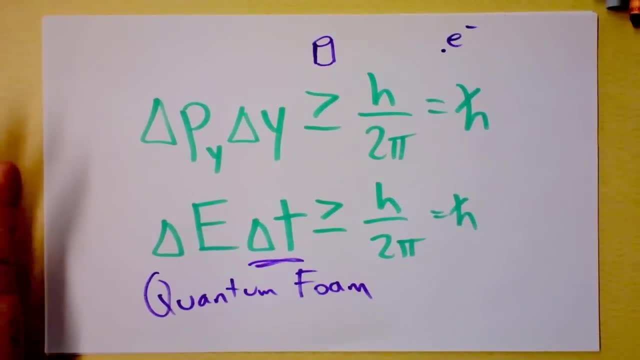 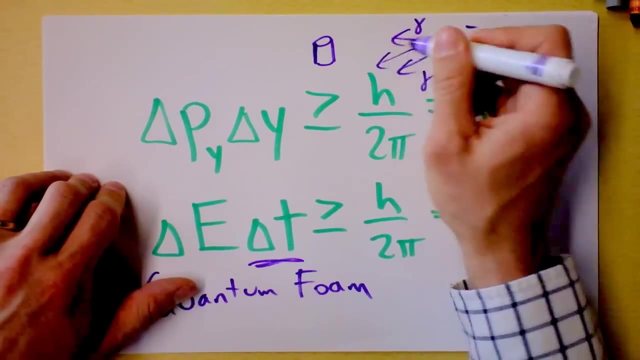 to know where it is right. So you're looking at the electron. Now, what does it mean to look at the electron? It means that the electron must be reflecting some photons to your eyes Every time. you want to shine a light on that electron, you want to shine a light on this electron, you want 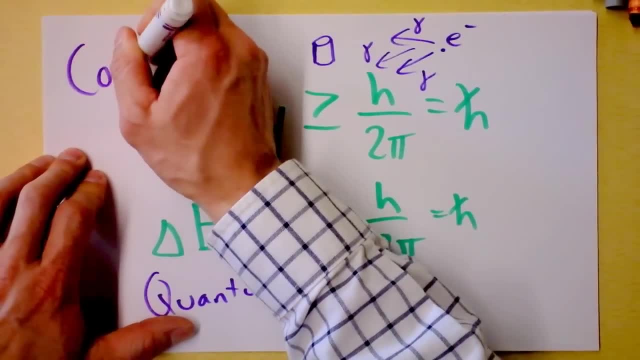 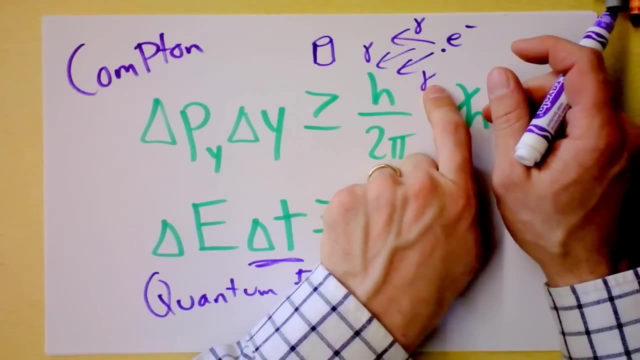 to hit this electron with a photon. That's what Compton did, And you know what Compton found? He found that that electron would go some crazy direction as a result of its interaction with the photon. The only way to observe a system is to change it in. 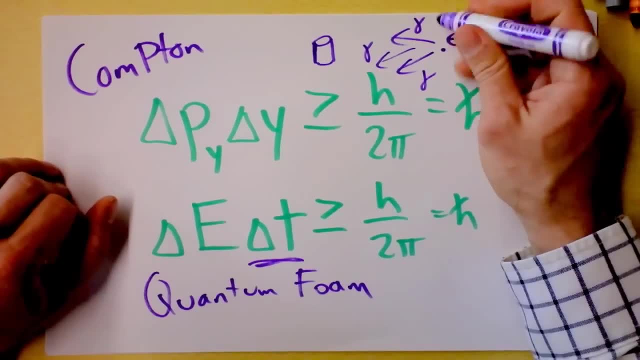 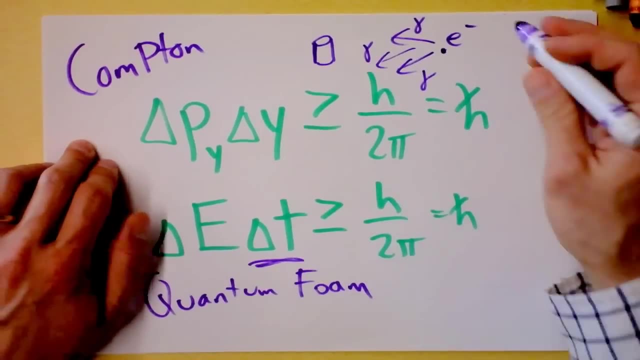 the act of observation And, in fact, the more accurately you want to know the position of this electron, the higher energy photons that you must send to it, because the higher energy photons have a. let's see, energy is h times f. the higher energy photons have a higher frequency than the. 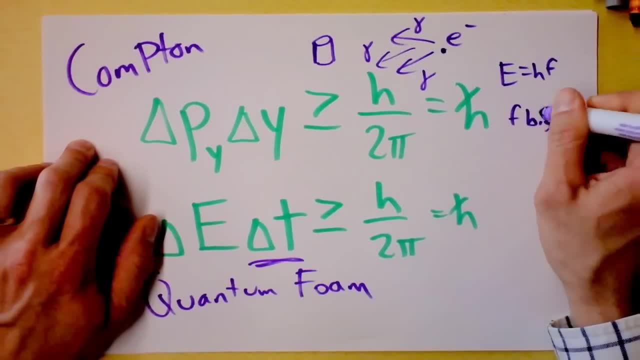 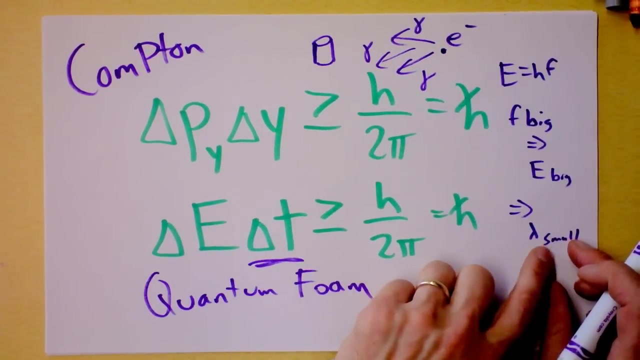 electron, which means that let's see, f big implies e big, which implies that the wavelength is small, which means that you'll be able to very accurately know where the electron was. But the more energy you send in to hit this electron, the more you're kicking it. who the heck knows where. 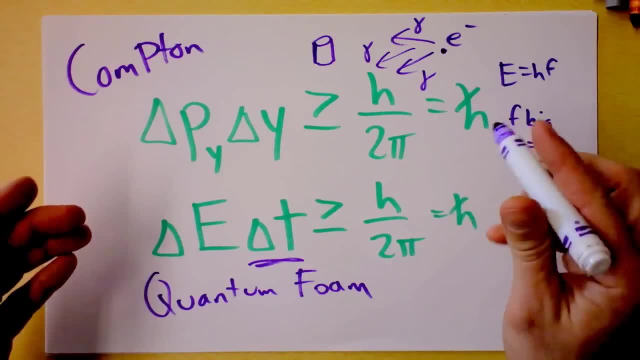 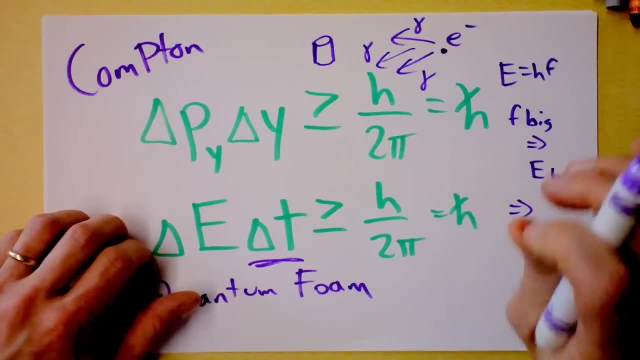 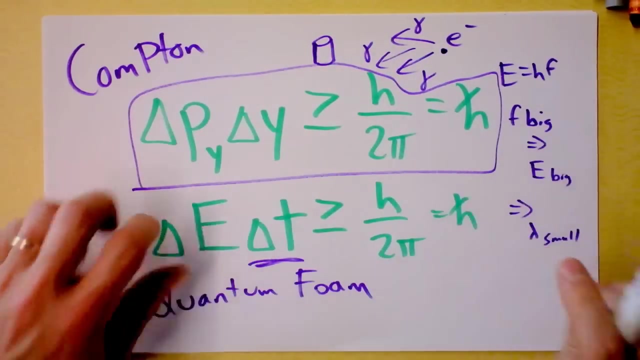 Not just you don't know how fast it's going, you frankly have no idea which way it's going. If you know where an electron is, then you suddenly have no way of knowing which way it's going. That's what Heisenberg is saying to you. It is not just a special case of observing electrons, or this. 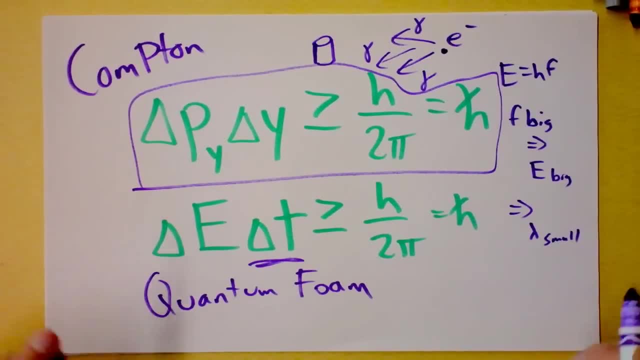 double slit thing or single slit thing. It's real, it's deep and it's fundamental. It's very, very interesting physics.